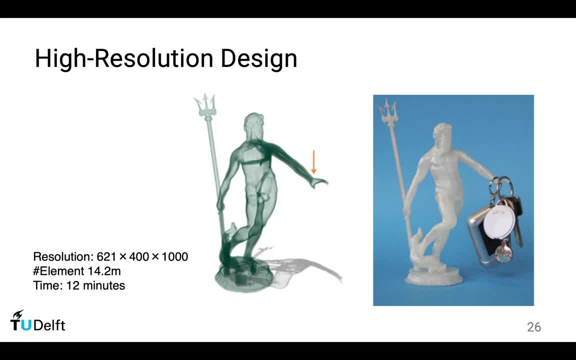 from a few hours, or even a few days, to a few minutes, which is significant. this brings topology optimization from a tool only applicable to aerospace and automotive industry to consumer products, so we hope to bring this to even at real time. so for the design of consumer products or even customized products, you can play with it. 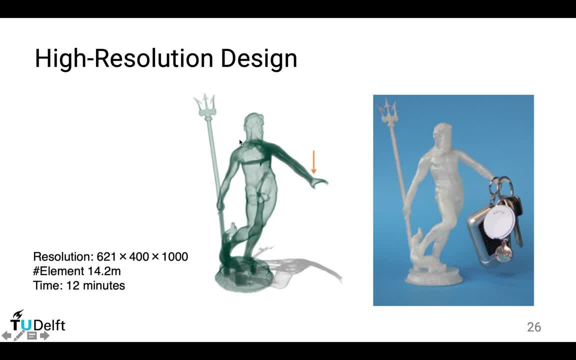 so this was the research we did four years ago. we applied it to design this internal structure or the support structure in the statue. forces applied on the hand and you could observe the head and the tripod. they are empty because, apparently, force is not transmitted to this region. 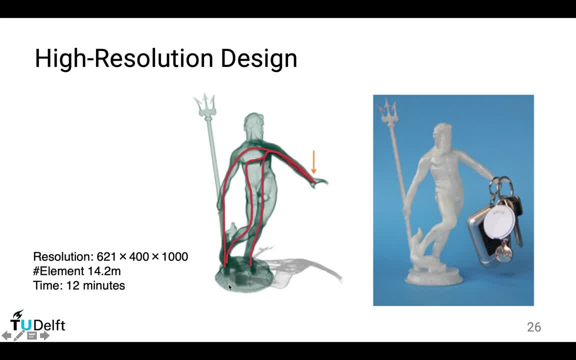 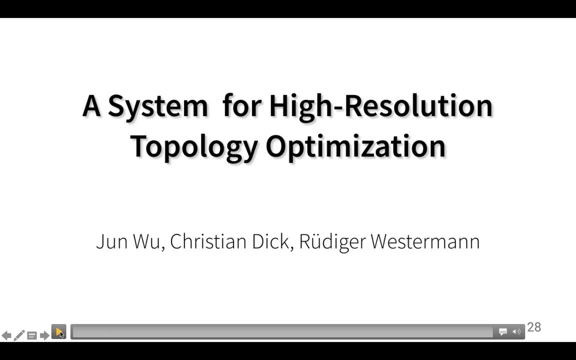 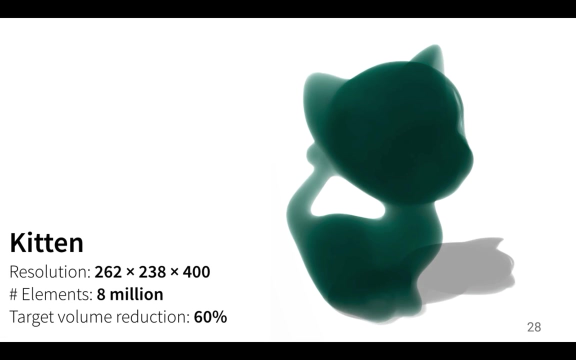 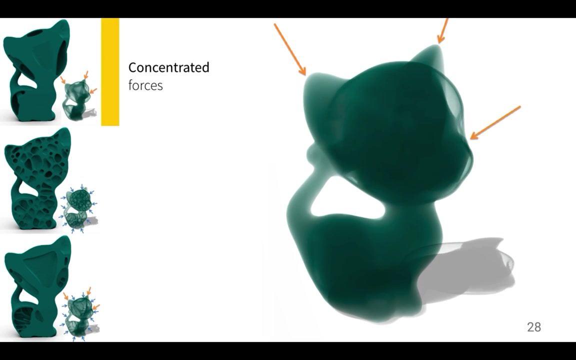 it transmits through through three passes to the fixation on the ground and on the right hand side is fabricated with fdm printing. this video shows a few more examples of 3d topology optimization. let's have a look. so the optimal structure is adapted for different forces. very interesting if we have a distributed. 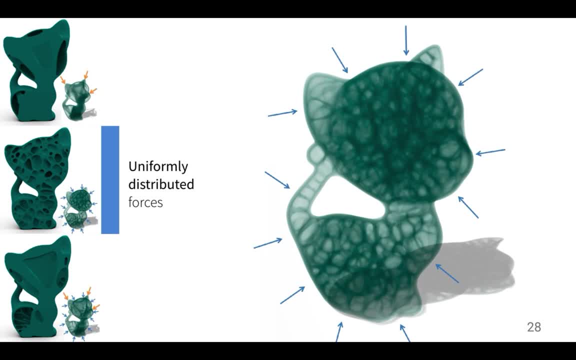 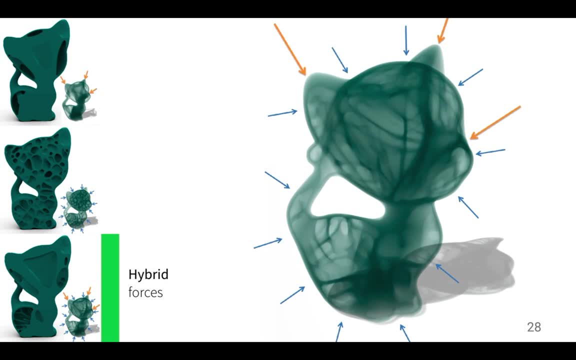 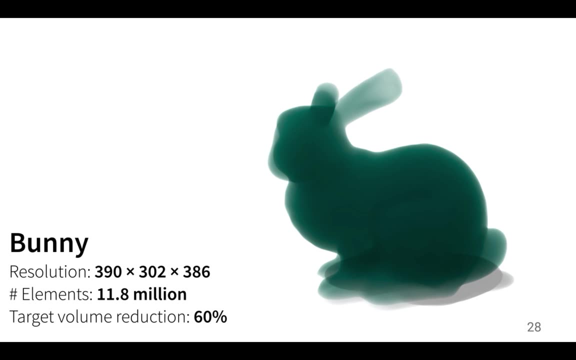 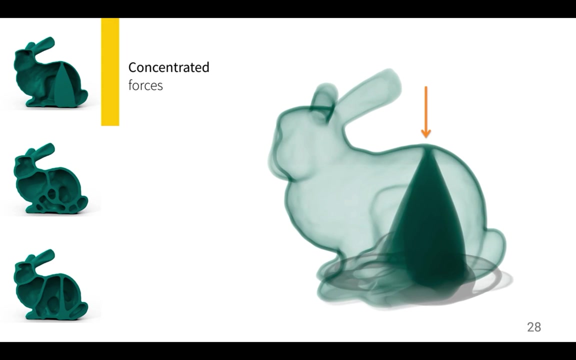 load we observe many bubbles and this is a combination of distributed pressure load and the three concentrated loads. we also have a different model with 12, almost 12 million elements. so this is a combination of distributed pressure load and the three concentrated loads. again with the pressure load we have very interesting bubbles. i like it very much. 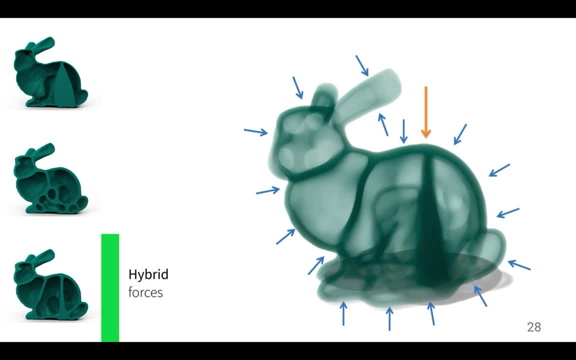 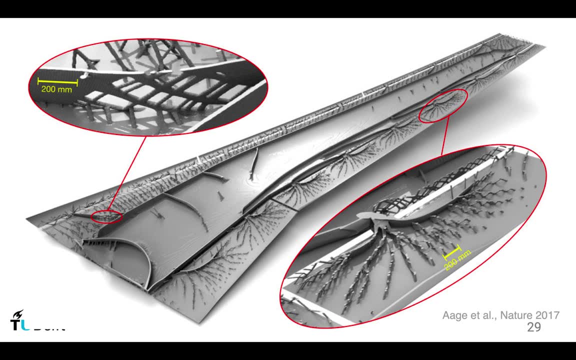 and then this is a combination of distributed load and concentrated load. my colleagues at the dtd Denmark make a step even further. they simulate the entire airplane wing with extremely high resistance to the wind, with a higher angle resolution. so here they have a few billion finite elements. 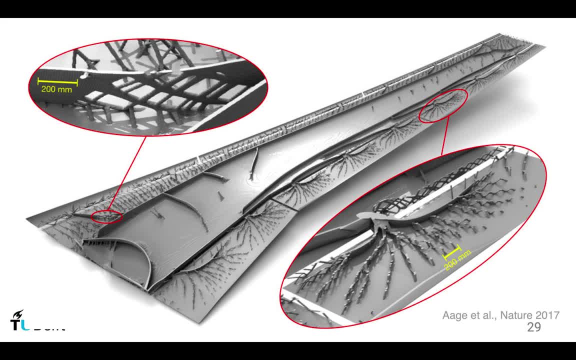 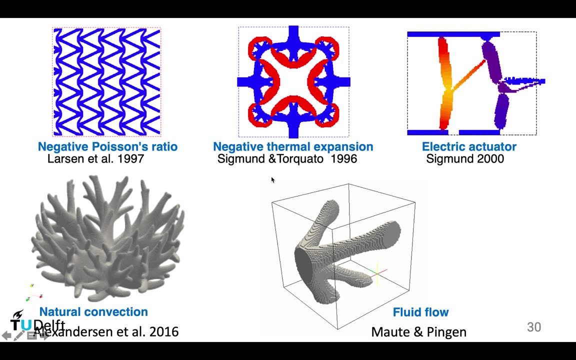 and at this scale, they could come up with a detailed optimized geometry. and this research was published in nature in 2017. topology optimization. so until now, the examples: the chair, the airplane wing, the K10. they are optimized for stiffness. Topological optimization also applies to 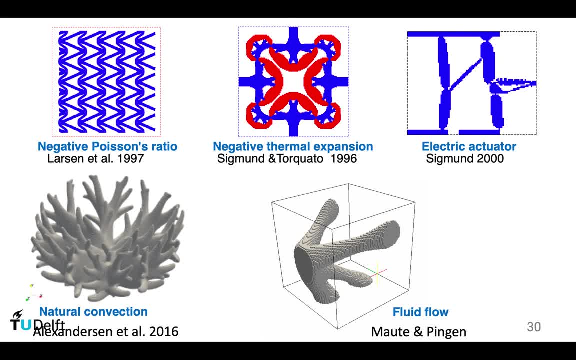 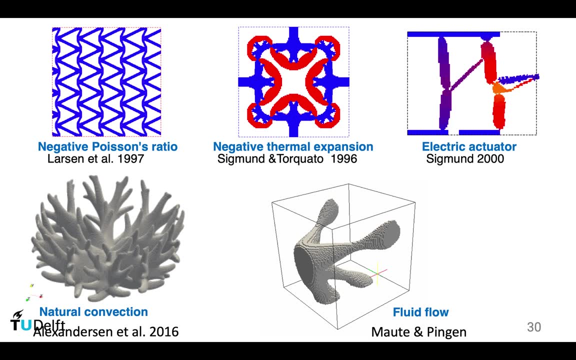 other physical phenomena for different mechanical performance measures. These five examples I selected to explain to you that it is a very versatile process applies to many different physical phenomena. On the top left it is optimization of material with negative portion ratio, which is also called auxetic material. Normally the material has a positive portion ratio, which means, if you 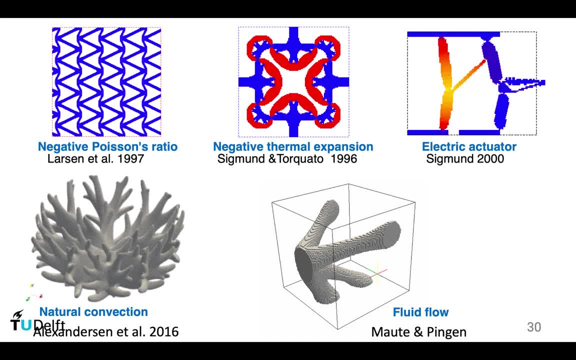 compress the material in x direction, it will expand in y direction. This is normal, this is as expected. but with negative portion ratio, you compress along x direction. it also shrinks in y direction and this is counter intuitive By designing microstructure or architectured geometry. if you consider this block as a material, it has a negative portion ratio. 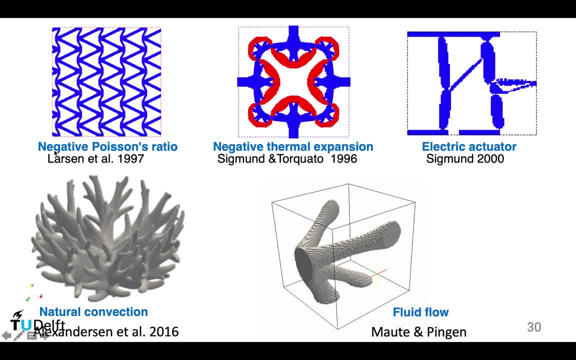 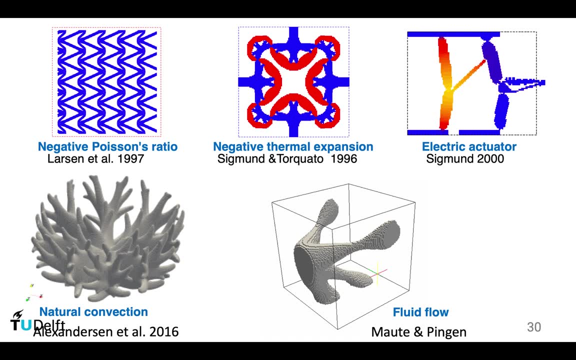 Let's have a look at this animation. Now. if you look at this animation, if you compress it in the x direction, the y direction is also compressed or shrinks The applications. my colleagues have been applying this negative personalization material to the design of implant and also personalized cast, so the cast could grow with a boy or with a girl. 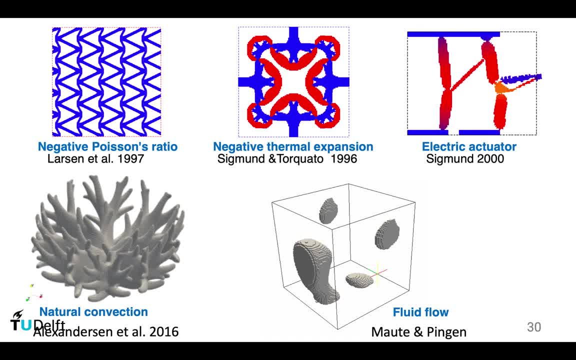 in all xy directions. The one in the on the top middle is the design of metal materials with negative thermal expansion rate. Most material we find in nature. they have positive thermal expansion rate. You increase the temperature, it will expand, the volume will expand And here, by placing two materials, these two materials have different. 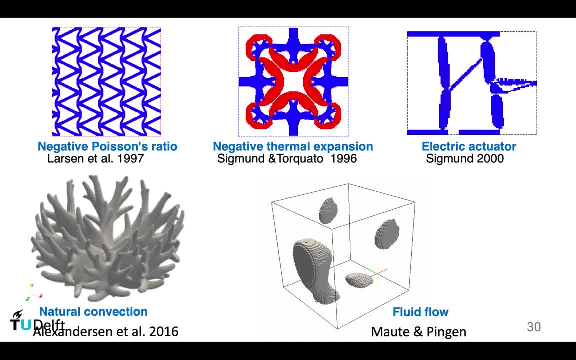 thermal expansion rate. When the temperature is increased, some parts shrink and as a block, if we consider it as a material, effectively it shrinks. So this is a negative thermal expansion material. On the right hand side is an electrical actuator. It is designed to move first to the 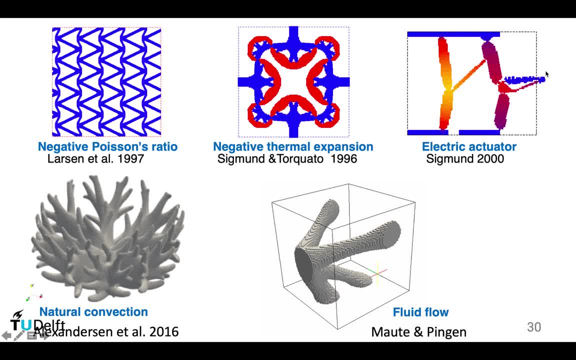 right hand side, Then upwards. This is very useful for MEMS At a small scale. it's very difficult to assemble structures, So it's good to have the actuator in one piece, And here is a compliant structure in one piece, actuated by electricity. So it 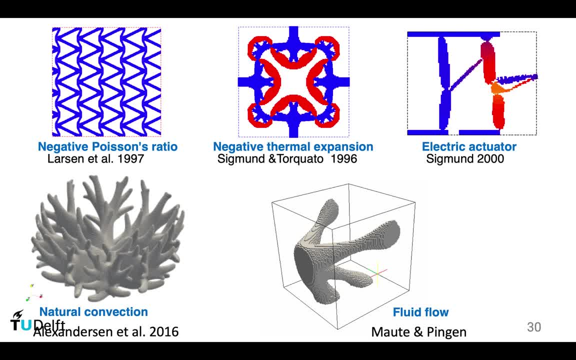 makes assembly not necessary. On the bottom left it involves natural convection. So the purpose is to dissipate heat from the middle to the outside as much as, as fast as possible. Think of heat sink in your computer. And on the right hand side is optimization regarding fluid. So the fluid will flow from this. 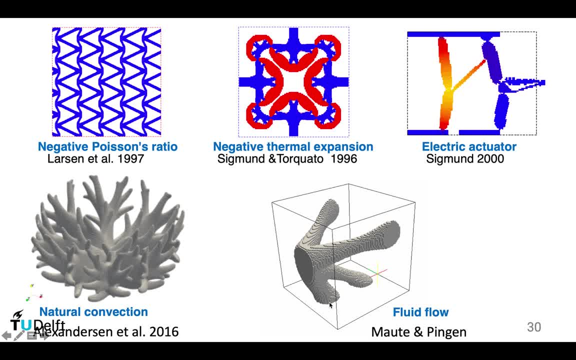 port, And then there are four outlets. Here the objective is to reduce the pressure drop as much as possible. So, as you see, topology optimization is a very general idea. It discretizes the domain into elements and it optimizes the material distribution within its design space on a per point basis. 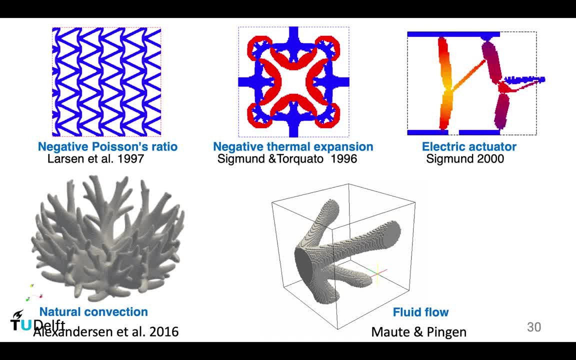 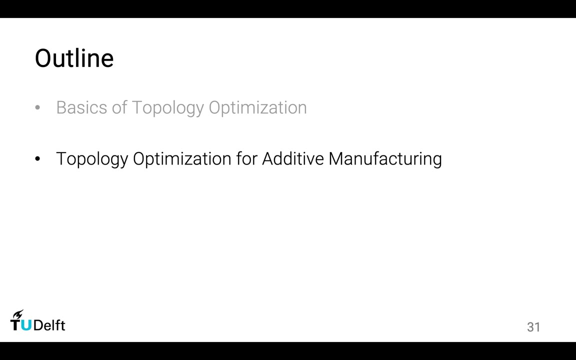 And in the design of many products, the geometry would influence the performance regarding the physics, and if this is the case in your project, you could consider topology optimization for your, for the design, for the automated design. so this is the basics of topology optimization. we will have a break after. 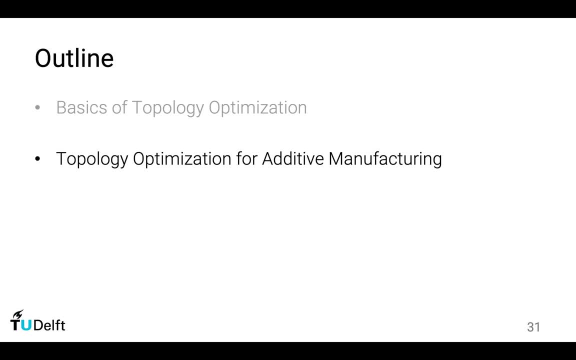 this break, we will particularly look into additive manufacturing. regarding the challenges and opportunities,